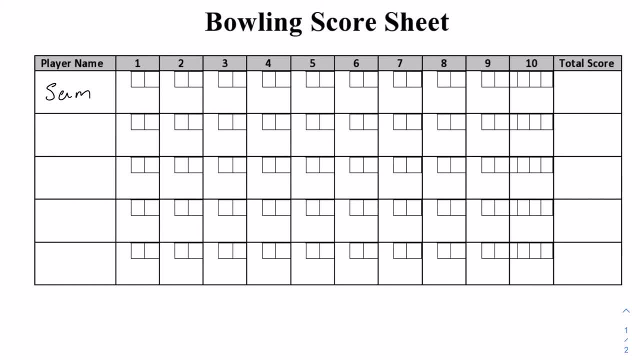 i think i'm going to do two different scenarios just to see how the scoring works, depending on what happens. depending on what happens and what the bowler throws. so we're going to do sam and we are going to do oliver as our two people. so i'm going to start off with sam and we're going to 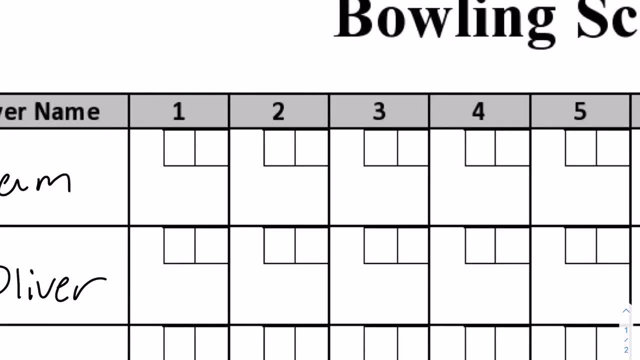 go across the line for sam and then i'm going to go across the line for oliver. so we're just going to say for sam, their first throw is an eight and their second throw is a one. so what you do if there's just two numbers in the box, you just add the two numbers together and you get the points as 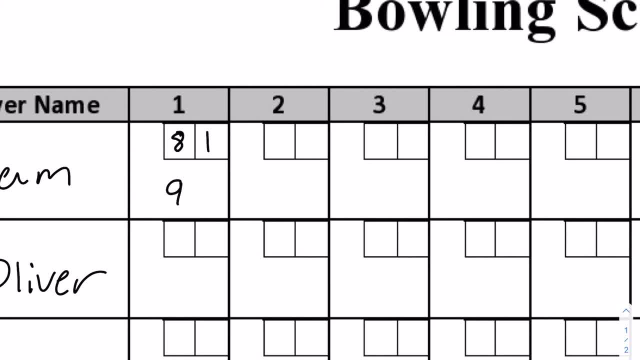 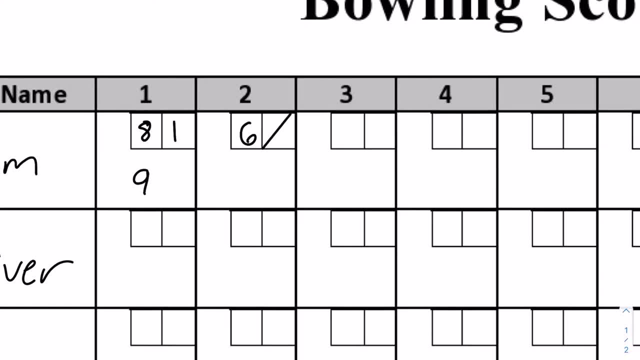 nine. then on the their second throw they're gonna get a six, and on this one they are able to actually get a spare. so they got the other four pins down. so you draw a single line through that box. now what that means is, because they got a spare in that box, you are not going to put anything in the box below. so 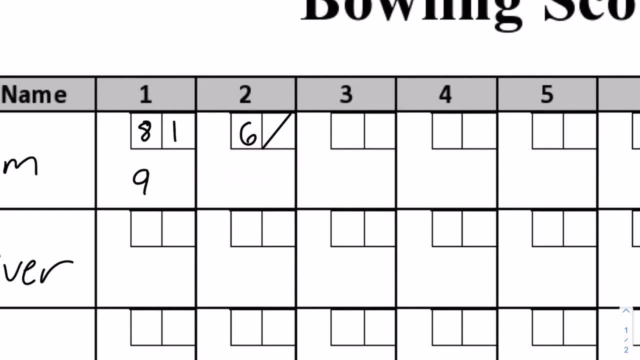 you're going to leave right here nice and blank, but you are going to then roll the next ball. so when they bowl the next ball, say they got an eight. so the important thing to remember is for a spare you count the next ball after. so the spare is 10 points plus the following ball. so for this you get 18 total points. when you add 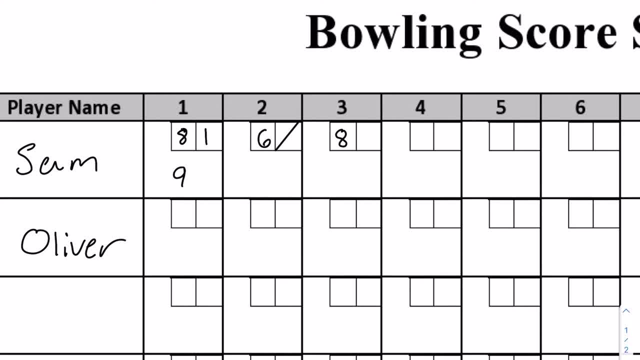 the 18 to the 9. you are then going to get a score of 27, so you're going to put 27 in this box. after that they bowl again and they get another spare, so you're going to draw another line. you are then going to roll again. we'll say: we got a four this time. not as good, so for this you. 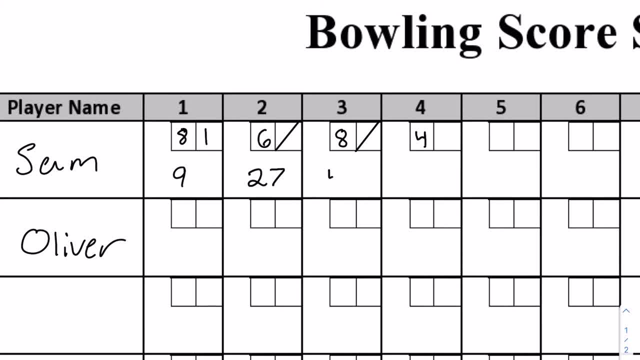 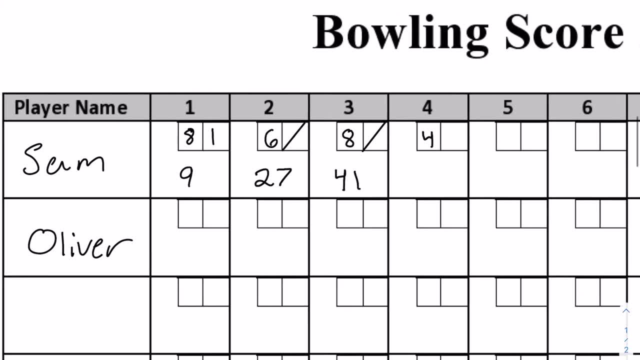 have 14 as your total. so when you add 14 to the previous square you get 41. so what you are doing is you are adding the total for round three to round two. so this total because of the spare, you do add that next ball as well, and then for this let's say they get a gutter ball, just not a good. 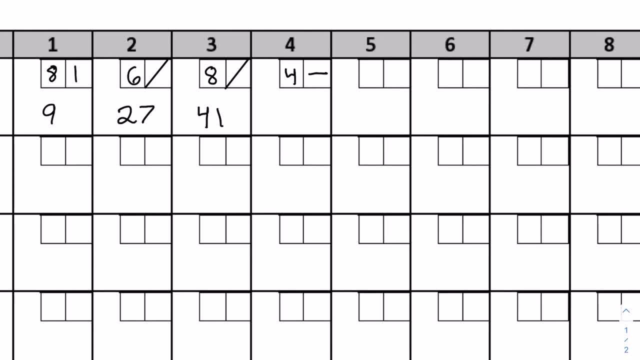 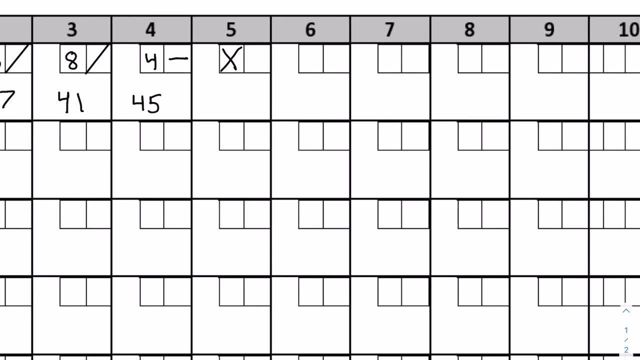 frame for them. so you add another square to that next ball just to make sure they are going to roll. add that four points in and they are now at a 45. Following frame. they get a strike. So a strike is written as an x Big thing to know. with a strike you can actually remember this. an easy way to. 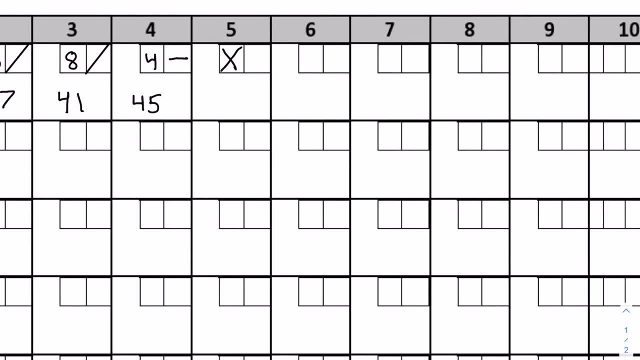 remember this is with the lines that you have to write. So because it's an x, it's two lines. that means you have to count the next two balls as well. So a strike is 10 points plus the next two balls. So for this one they get a strike. On the next frame they get a six and then they get a three. 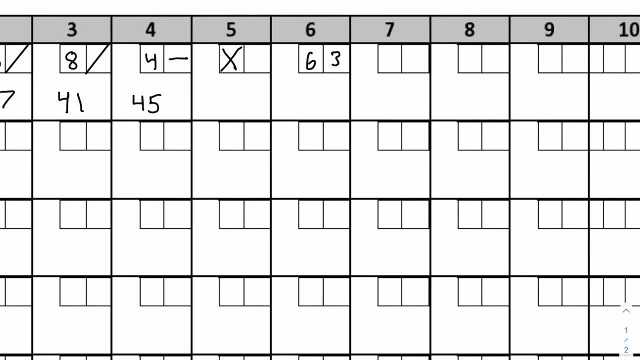 So they got nine points. So that means that total for the previous frame was 19.. So we're going to add 19 to our 45 and we are going to get a total of 64.. So 64 is their total score currently. 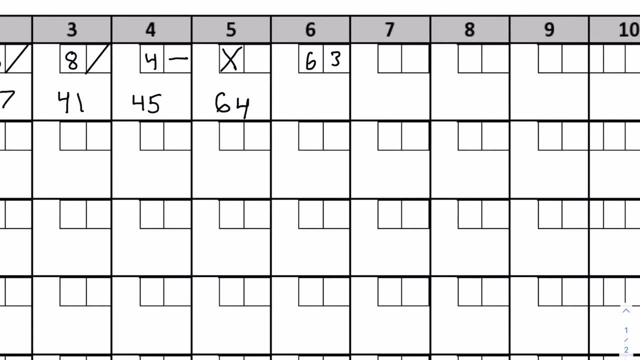 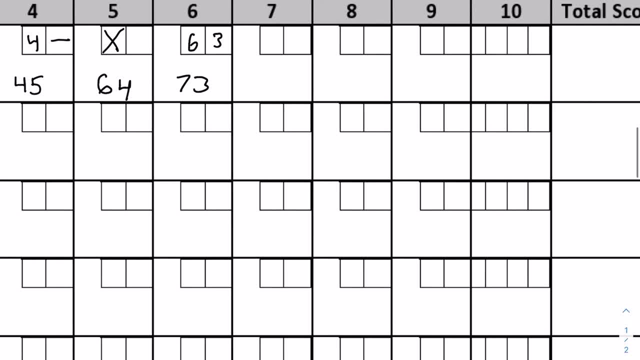 You're going to add in frame six. You can add in that next set of nine points. So to do that, you just add it right in To give them a total of 73.. They're going to bowl again. They're going to get an eight and then a. 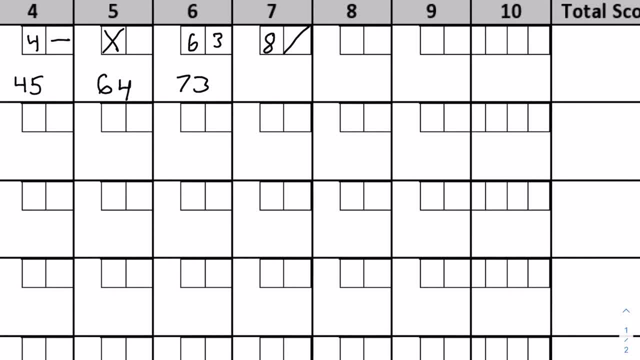 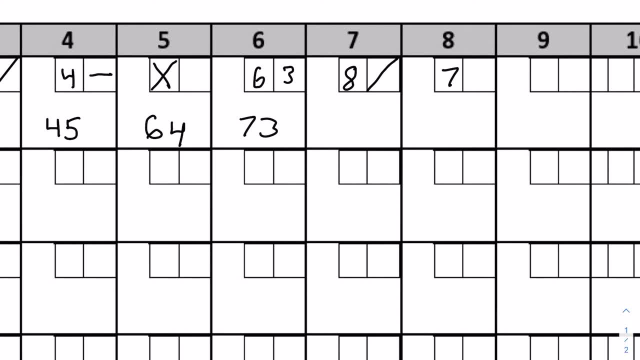 spare. So for this one you can leave it blank until you do the next one. We're going to get a seven. Now that they got that seven, we can add in that previous frame points of 17 to put us to an even 90. They then get a two to add another nine. So we're at 99.. In this ninth frame they get a. 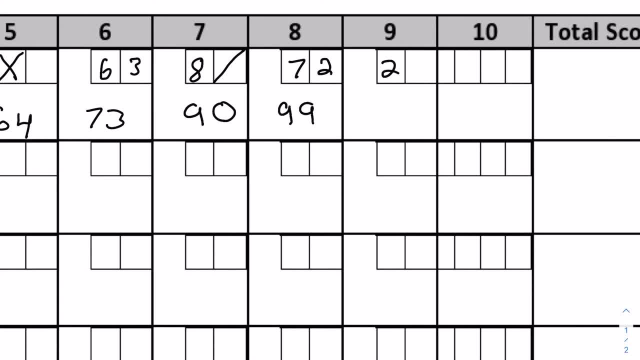 nine, They get a two, So not a good frame for them. And then they actually throw a gutter ball. For a gutter ball or a ball that doesn't hit any pins, you just draw a horizontal line. So this puts them at a score. 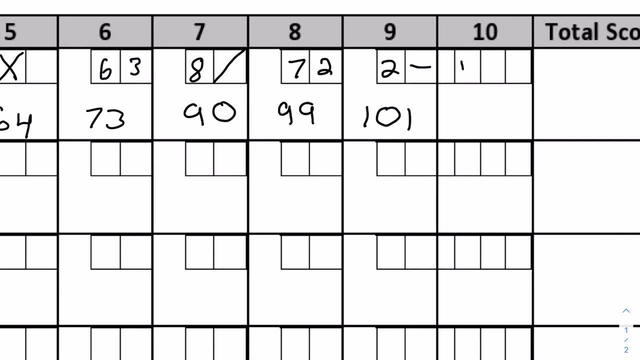 of 101. And then for this one they get a five. Now, one thing to remember in this 10th box, because you are guaranteed those two extra balls after a strike, or one extra ball after a spare. you may throw up to three balls in this box. So what we're going to do is we're going to get a five and then they're. 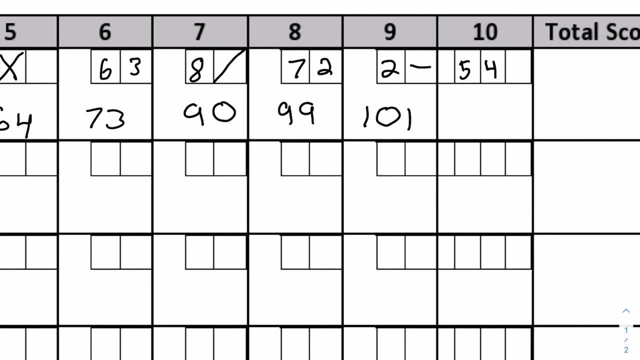 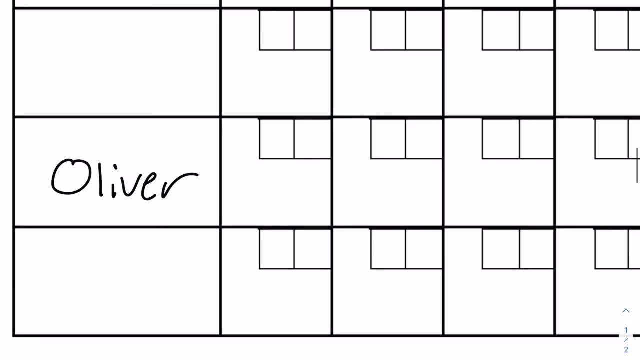 just going to get a four. So they're going to end with that For the seventh to ninth to give them a total score of 110.. So you put in this final box 110 as their score. I moved Oliver down so we could separate out his score. so for Oliver Oliver is he much more experienced? 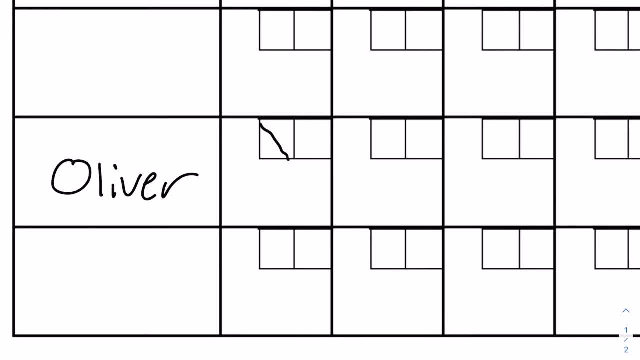 bowler. So for this he is actually going to start off with a strike. So that means we have to count the next two balls while Oliver gets a strike for the next round as well. So that's ball number one, and then the following one. 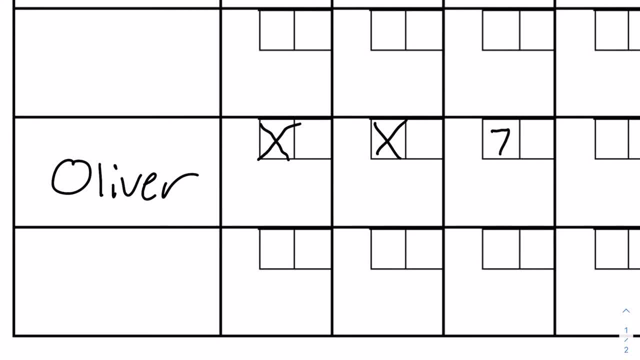 He gets seven. so for that first frame oliver has a score of 27.. now, moving on to that second frame, we need to remember it's two balls. so for this you count. you have the 10 from the initial strike, you have a 7 in the next square and then the next ball he rolls gets him a spare which totals that to 10. 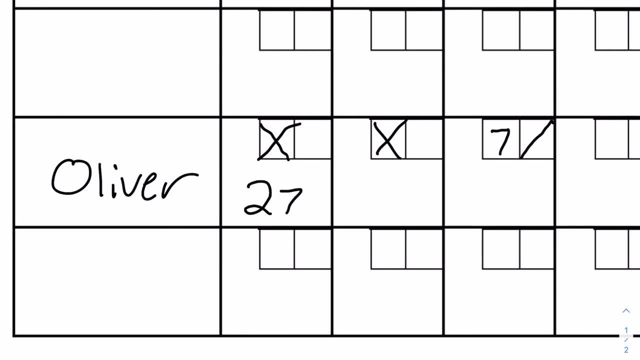 which means 20 is the total for this next one, so which makes him a total of 47.. this one i'm actually also going to switch back and forth between colors to show that the this is a 20 point addition. so the red numbers are gonna be what we're adding together, but the black number is. 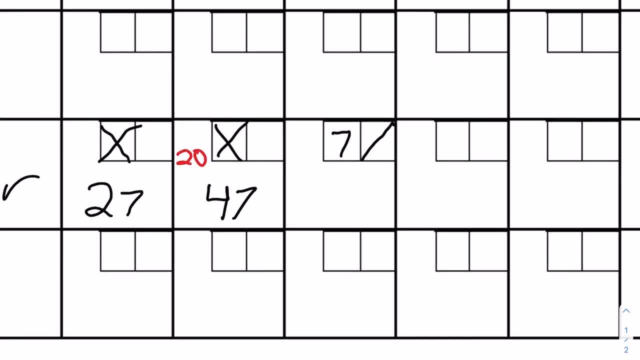 gonna be keeping that total score then sliding over. on the next frame. we have to throw another ball and for this one he throws an eight. so for this we have to add up the score for the previous one, because it's a square, so he's only pulling 8, so that number is 8 and i'm gonna stack all of these. 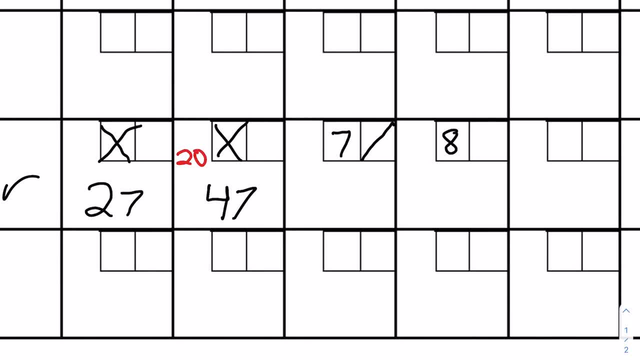 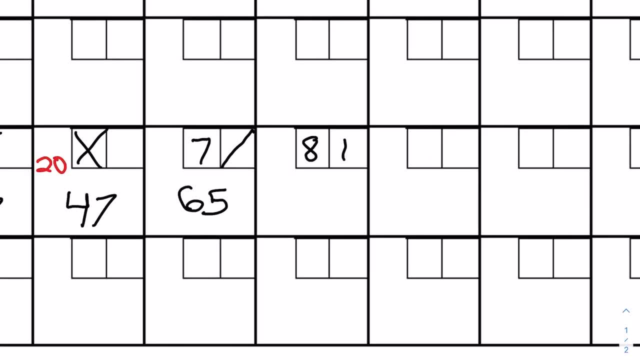 igt ones up. so i'm going to add 2 to each number and start throwing that score. and then, hogyavind, it was a spare, you have to have that extra ball. so for this one you got a score of 18, which puts oliver now at 65. then got a one which adds a total of nine points to put us at a score of 74. 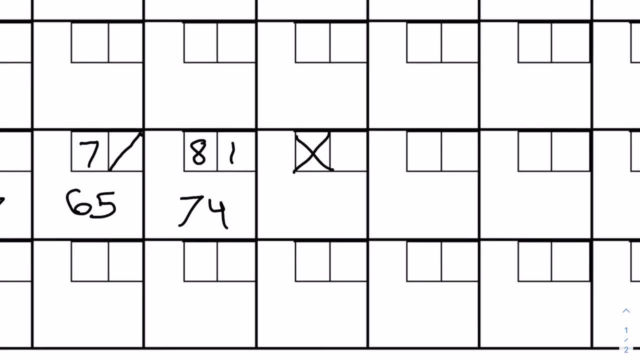 oliver then gets a strike. remember you got to count the next two balls after that. so not a good throw after that, which is a four and then a two, so just not a good frame for oliver. you then add in: okay, you have 10 plus four plus two is 16. adding that to our 70 gets an even 90. now the 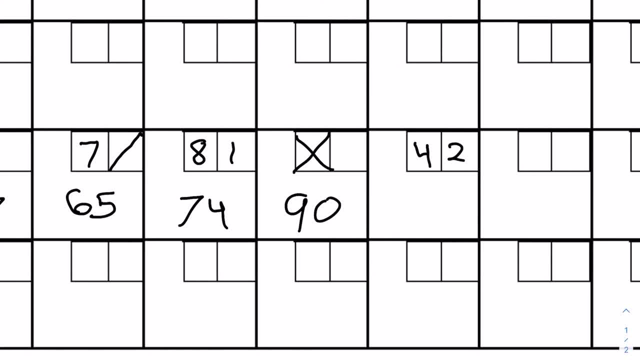 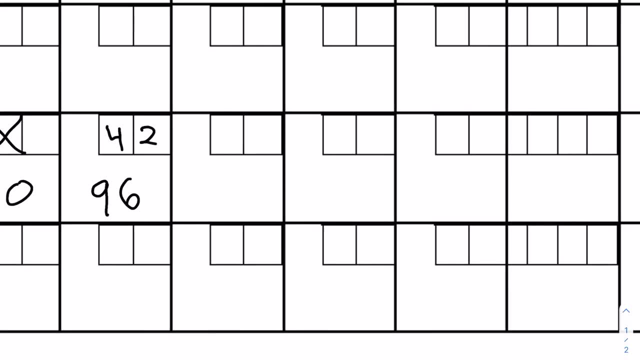 big thing to understand with a strike versus a spare. for a strike you have those two extra balls to score some big points. for a spare, you really want to score some big points in that next throw. so now we add in that extra six points, so we're at 96. we got a another round with a five and a. 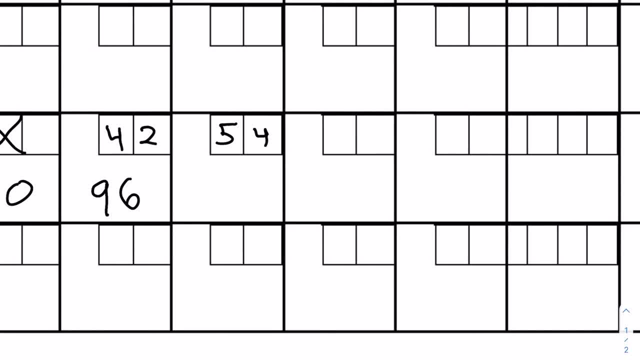 four, two, three get us to another nine points, which puts us at 105. we then have a throw of seven, and then you get down those last three pins and end up with a spare. then we have a throw of nine, unable to capitalize on that last one. so we just leave that last one blank. so with that nine we add that 19. 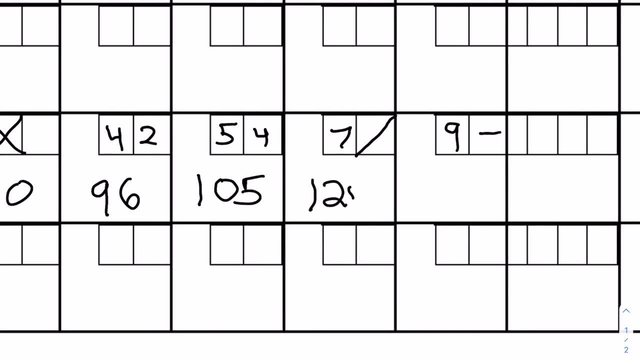 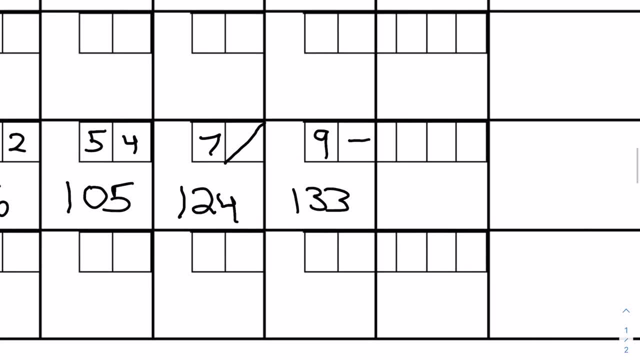 points, which puts us at a hundred and twenty four. we add in that other nine to put us at 133. going into this last one, oliver does throw a strike and then actually throws a second strike and then throws a seven. so for this one he doesn't get any bonus, for that second strike he doesn't. 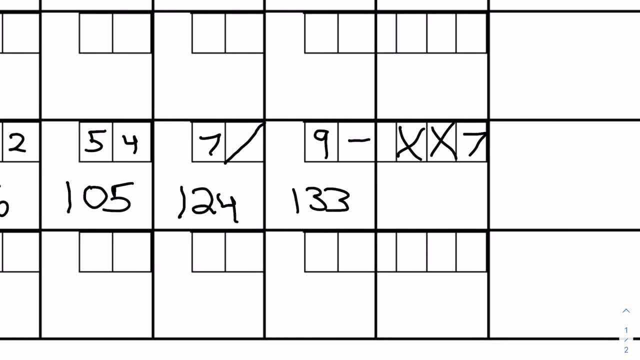 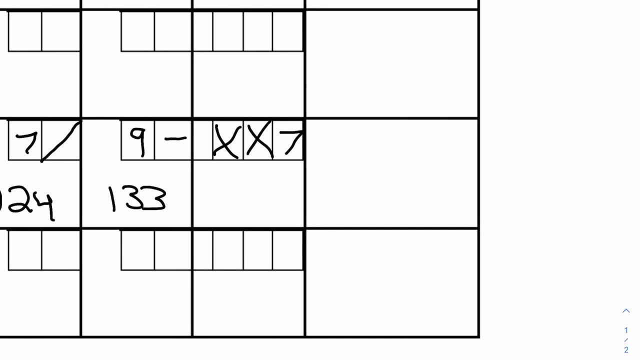 just keep throwing until he misses or any of that. so you just add these two together to get 27 out of 7 points, the score for that last one, and you have a total of 27 plus your 133 to get you to 160.. so we just 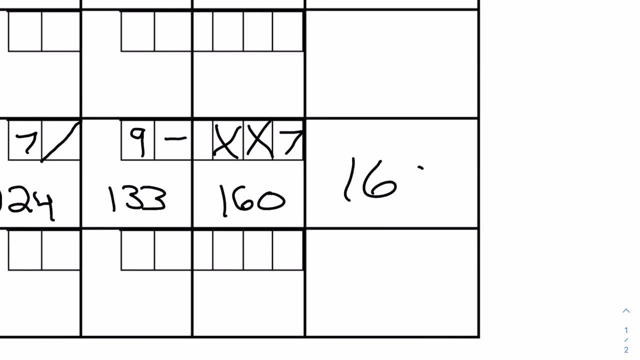 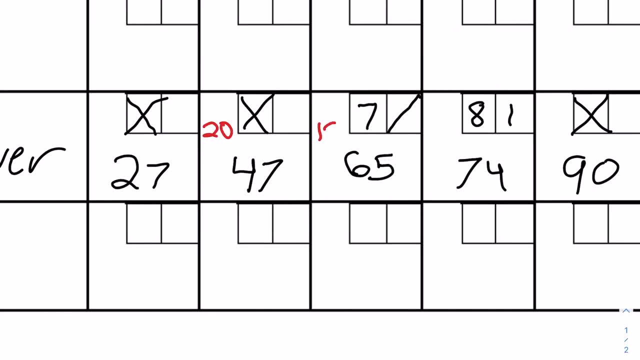 add that together we get 160, and 160 is the final score, just going back. i'm going to write in those red numbers so you can just see those as well. for this one we are adding a total of 18 points. for the next one, we were adding nine. 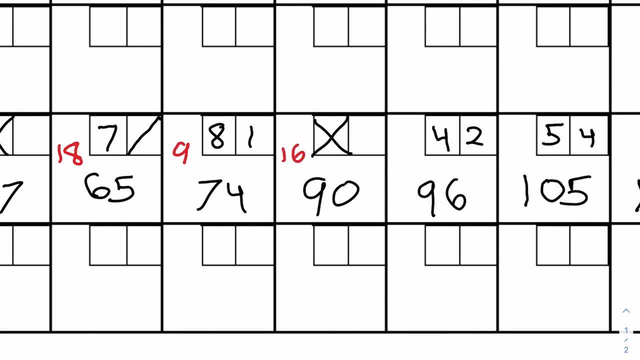 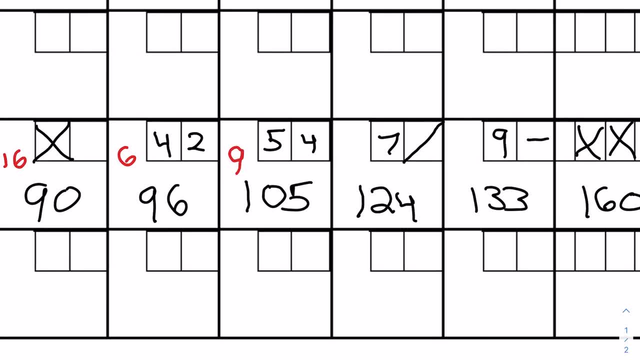 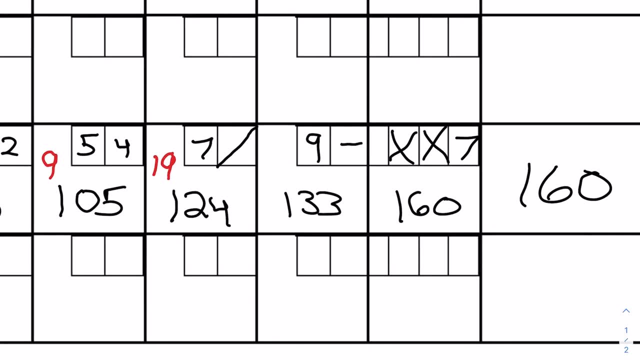 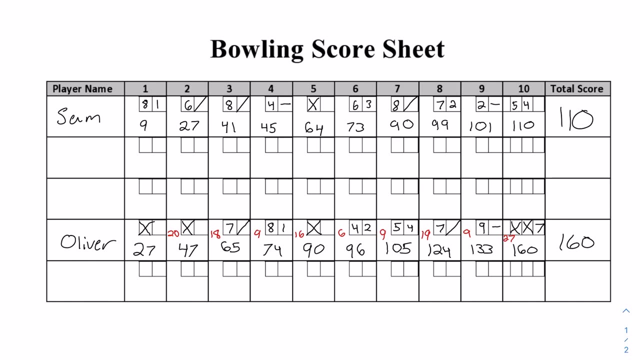 for this one we were adding 16, we then added six. after the six, this next frame, we added nine, then we added 19, we then added nine and then for this final frame we added 27.. so showing the full score sheet, you can see that those red numbers. they show off all the different ads that you did for this. 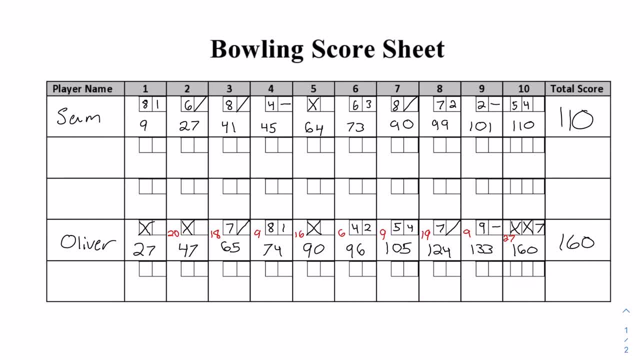 so you have olive's full 10 frames, you have sam's full 10 frames and you can see, adding those strikes and spares and getting those extra bonus points in the next frame do help build your score up. but that is the basics of a bowling score sheet. if you have any questions, definitely let me know in.